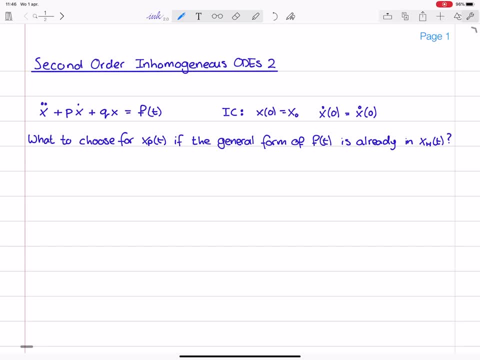 something that is already in the homogeneous solution. So this is never. in this way, it is never possible to generate a new independent function for the particular solution, and this is not adding additional information. So we need a way out for this specific case, and this is done by a method called variation. 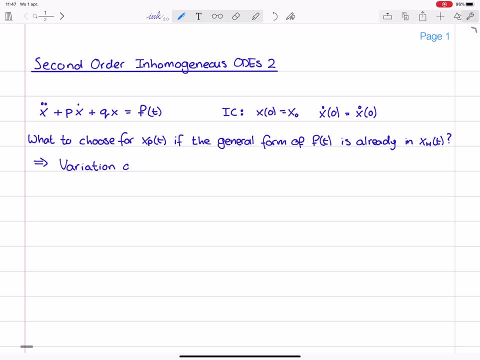 variation of constants, of constants. I looked it up and I looked it up, and I looked it up, and the Wikipedia page is called Variation of Parameters. but in the math book that I had when I was doing this ODE course, it was called Variations of Constants. 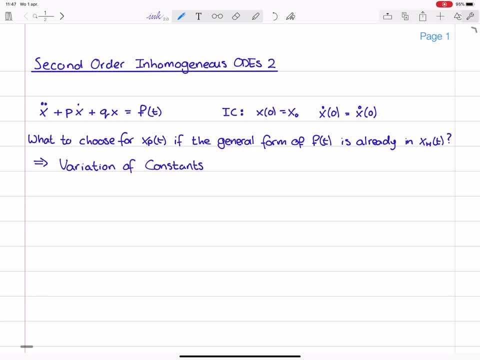 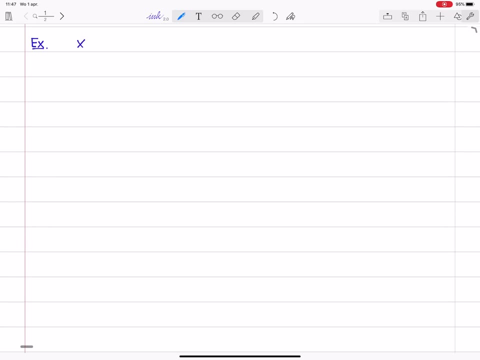 so that's why I will call it in this way. I will talk you through this method using an example, because I think that is the best thing, the best way to go. So for the differential equation, I will use the similar equation as what we used in the previous lecture on the left-hand side. 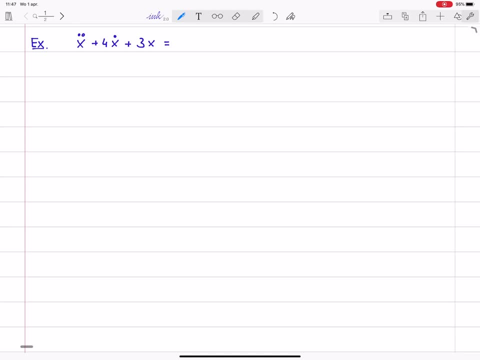 like this. and before I write down the right-hand side, let's recall the homogeneous solution, which was c1 e to the power minus t, plus c2 e to the power minus 3t. Okay, Now, in last lecture, 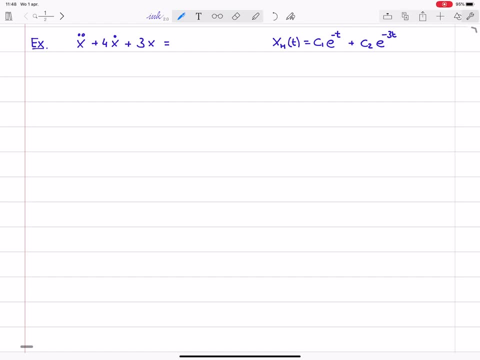 I showed you how to deal with right-hand side functions like linear ones, sines and cosines. but what happens if, for instance, this is e to the power minus t, Because now we would try for xp, for the particular solution, the trial solution. 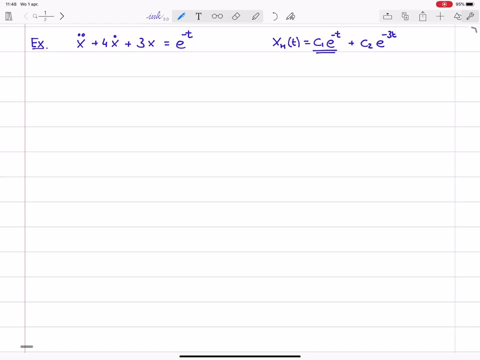 exactly this part right here. Okay, so when we use this trial function and we substitute it in the left-hand side, the result will be 0, and not e to the power minus t. So clearly this will not work. 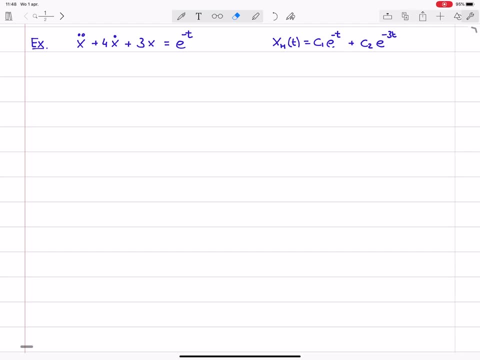 So this is a problem whenever the right-hand side is something that is already in the homogeneous solution. So the way out is as follows: We will try for the particular solution, the more general form of this homogeneous solution, in the following way: 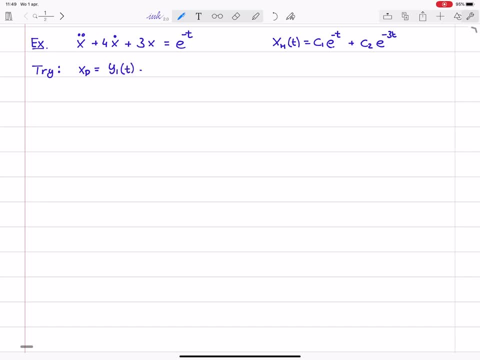 that we use y1, which may still be a function of time e, to the power minus t plus y2, which might also be a function of time times, this second solution. In a certain way, this looks a bit like the approach we had. 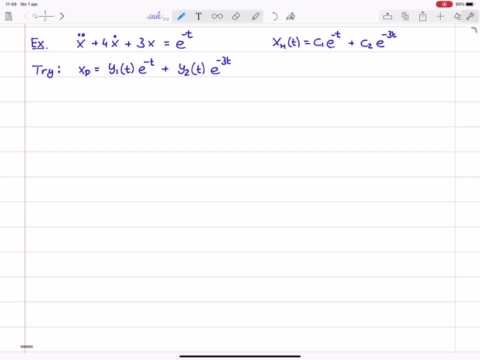 when we discussed the method of reduction of order. So I will allow for this coefficient c1 and c2 to be basically reduced and replaced by functions in time And let's see if we can construct functions for which this will work, And maybe this would give us an idea. 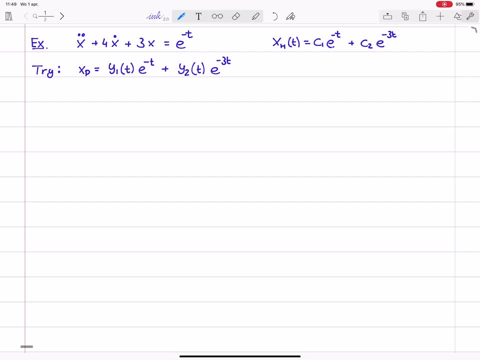 of what kind of function is a particular solution for this problem. So before we can substitute it, I need the time derivative and the second time derivative as well. So upon differentiation, we have y dot times, e to the power minus t. 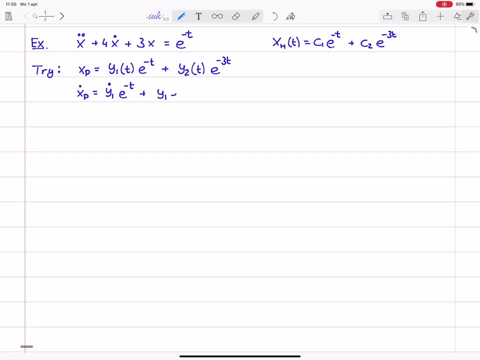 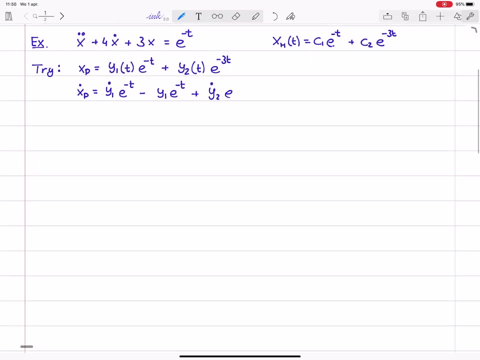 plus y itself, times e to the power minus t, and then times minus 1, so this becomes a minus sign. And then we have y2 dot times e to the power- oh, I'm sorry, e to the power minus 3t. 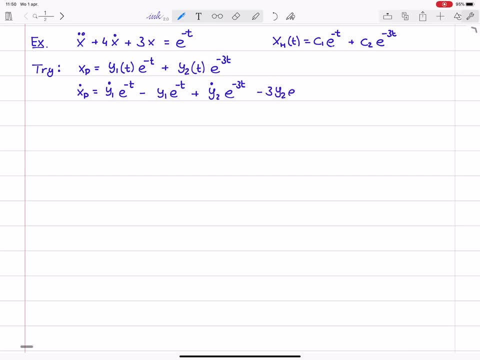 minus 3 times y2, e to the power minus 3t. So because I'm going to look for y1 and y2, so two unknown functions here and I only have to satisfy one ODE, I have still some freedom. 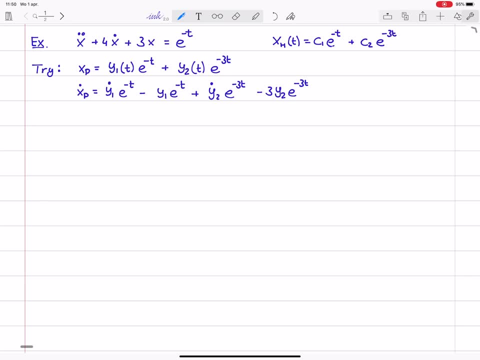 in how to choose y1 and y2.. And I will make use of this freedom at this stage because I will choose y1 and y2 such that these terms will cancel. This will greatly simplify the remainder of the procedure. So y1 dot e to the power minus t. 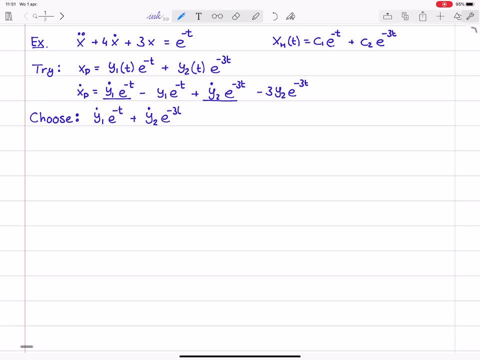 y2 dot e to the power minus 3t, I demand that this is equal to 0.. And I can do this because I have this additional degree of freedom. So as a consequence, we could say that, well, y2 dot is equal to. 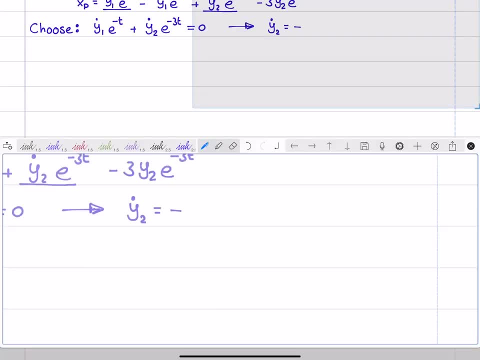 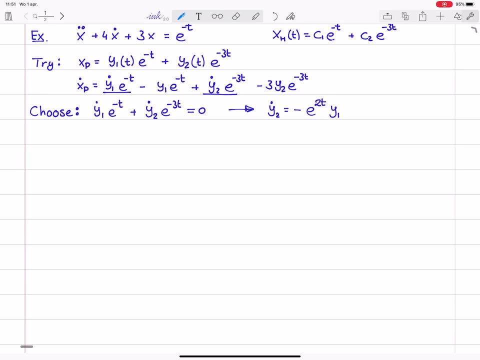 minus e to the power, e to the power, 2t times y1 dot. Alright, So I will make use of this relation later on, But I will box it for now. use it later. So that means that these two terms: 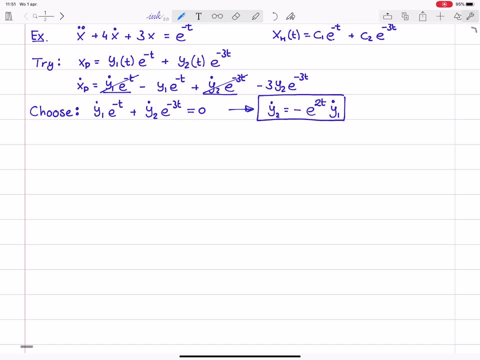 basically drop from this relation and that once we go to the second derivative we only have to differentiate two terms now, which become minus y1 dot: e to the power minus t and then plus y1, e to the power minus t. 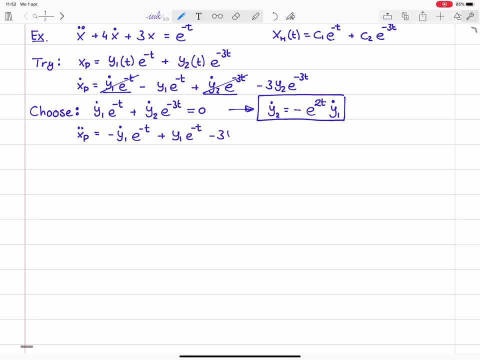 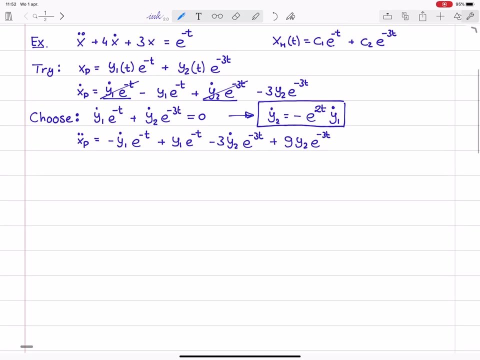 and then we have a minus 3y2 dot- e to the power minus 3t, plus 9y2, e to the power minus 3t. Alright, now I will substitute this trial solution for xp, XP, XP, dot, XP, double dot into the ODE and see what comes out. 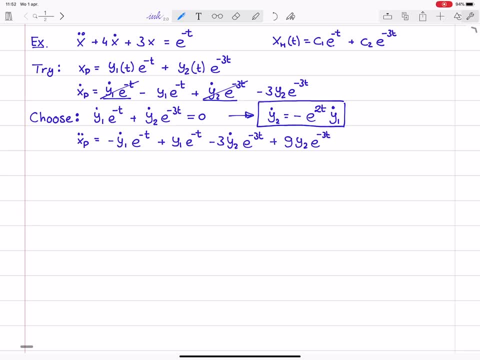 So I will start off by when we do this, you will see that there are terms produced with Y1, Y2, Y1 dot and Y2 dot. Let me first do all the terms that will be there with Y1 dot. 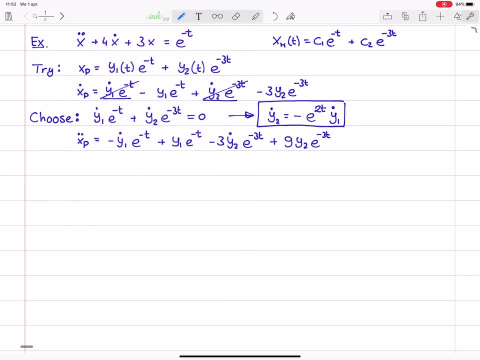 So this will be- let me maybe change color here- That will be this term. So we get minus e to the power, minus t times Y1 dot, And then we have the term with Y2 dot, that is this term over here. 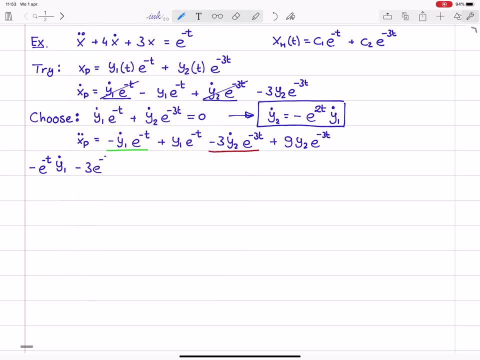 So that is minus three e to the power, minus three t times Y2 dot. And now I'm going to collect all the terms And then I'm going to collect all the terms with Y1 itself. So that is this one. So we have plus e to the power, minus t. 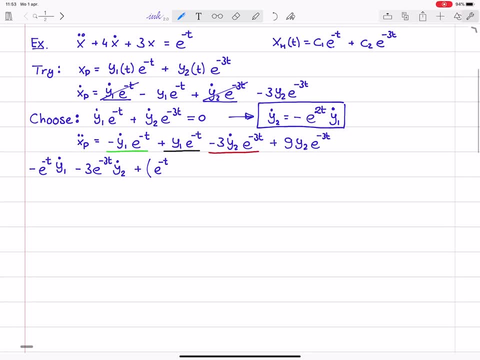 Then let's see, in the first derivative We have minus four times e to the power minus t. And then let's look at XP itself. Then we still have plus three e to the power minus t, So this term is null. Then we have minus two x y1 Elena. 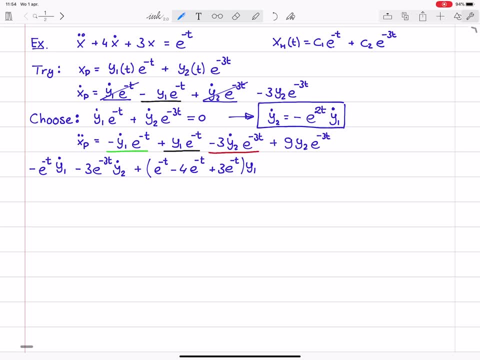 So plus three x y1, Elena. So I don't want to leave any space between the terms. This is a perfect equation. And then I can put this one in black, I can put this one in black, I can put that one in black. 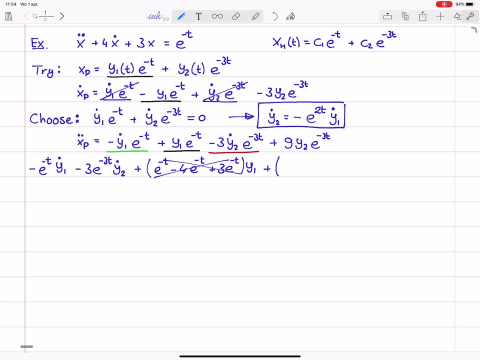 And then it should also be one plus one x y1.. Okay, so I have two x y1, Elena times y1. And then minus 12 e to the power minus 3t, And from xp itself, we have just plus 3 times e to the power minus 3t times y2.. 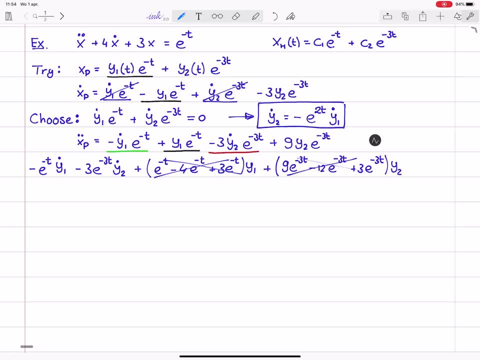 So also this term. in between brackets it cancels, drops out. That's good. So these are all the terms. This should be equal to the right-hand side, and that is e to the power minus t. Very well, So this equation greatly simplifies to: e to the power minus e to the power minus t. 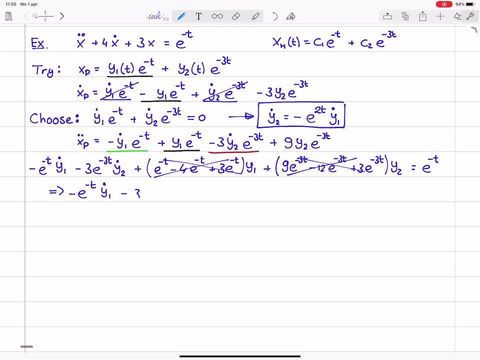 times y1 dot, minus 3e to the power, minus 3t times y2 dot, and that should be equal to minus e to the power t. All right, so this is a second equation for y1 dot and y2 dot. 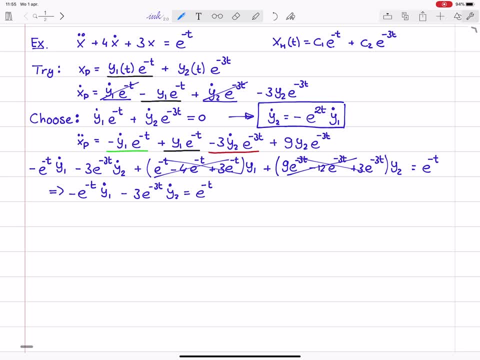 Let me at this point substitute the boxed expression the relation, The relation between y1 and y2.. Okay, so I get rid of y2 dot in this way. So we have minus e to the power, minus t, and then minus times minus is a plus. 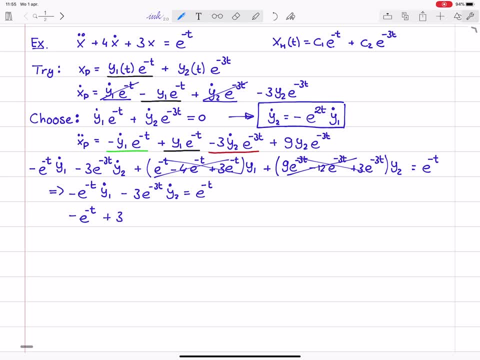 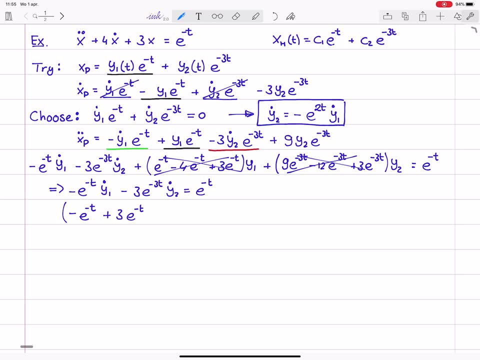 plus 3 times, and then e to the power minus 3 times e to the power 2t, that's e to the power minus t times y1 dot is e to the power minus minus 3 times e to the power minus t. 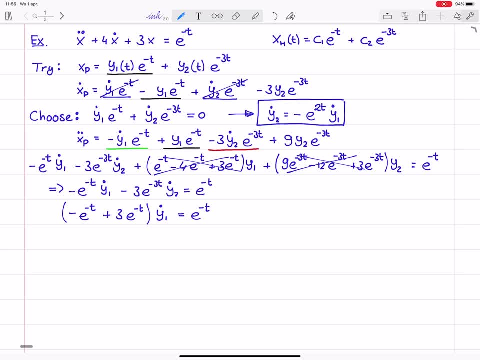 Good, so here we have minus 1 e to the power minus t plus 3.. So that is just 2.. 2y1 dot e to the power minus t is equal to e to the power minus t. So from this we get that y1 dot should be equal to a half. 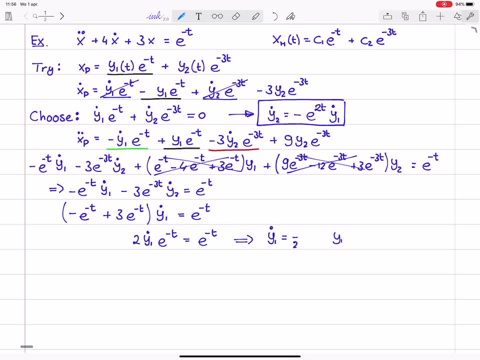 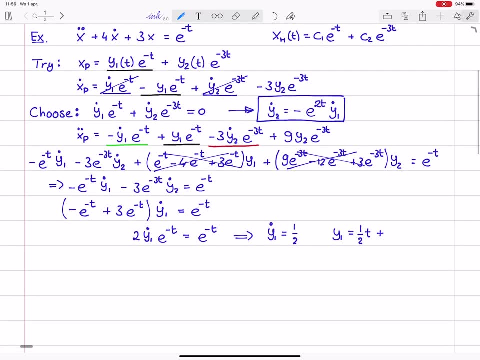 Great, So that's it. So that means that y1 is a half times t plus some integration constant. let me call that a1.. All right, so this is the solution for y1, the general solution for y1.. So we see, we try that. 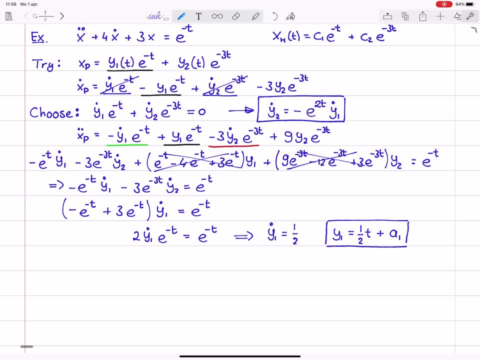 yeah, we use this trial solution where y1 and y2 are functions of time, and we see that indeed we manage. we manage to find a function y1 for which this works. And now let's look at the function for y2.. 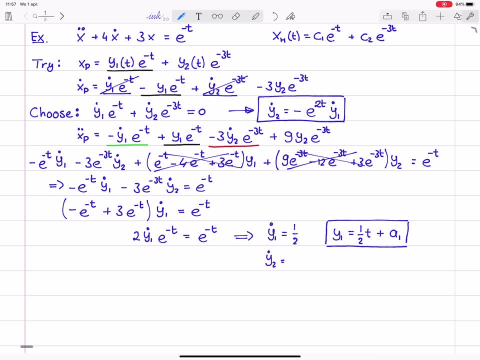 So y2 dot is minus a half e to the power 2t then. So that means that y2 will be: let me see minus 1 over 4 times e to the power, minus 1 over 4, e to the power 2t plus some integration constant that I will call a2.. 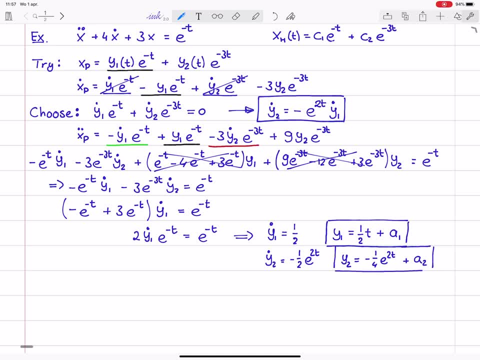 Good, So this is the solution for y2.. That means, if we now back substitute this into the particular solution, particular solution is: well, we have then 1 over 2 times t plus a1 times the first solution. that was e to the power minus t. 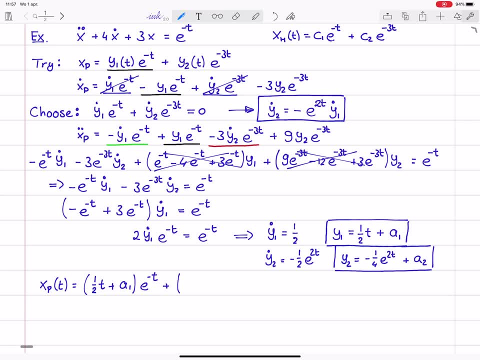 and then we have y2, and that is minus 1 over 4 times e to the power 2t, plus a2 times e to the power minus 3t. Very well, Now let's have a look here. If we look at this particular solution, 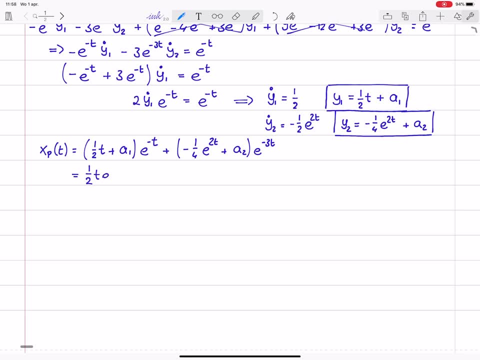 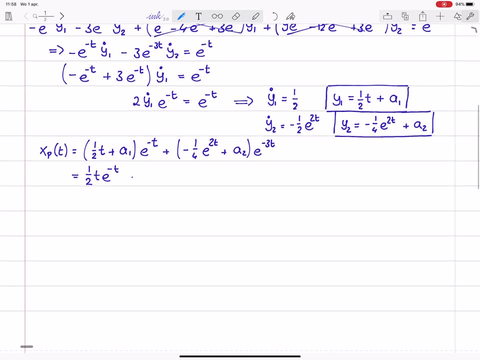 we find a term with this t in front minus a half t, e to the power minus t. and then we have terms with e to the power minus t itself, that is the term a1, and also this minus 1 over 4: e to the power 2t times e to the power minus 3t. 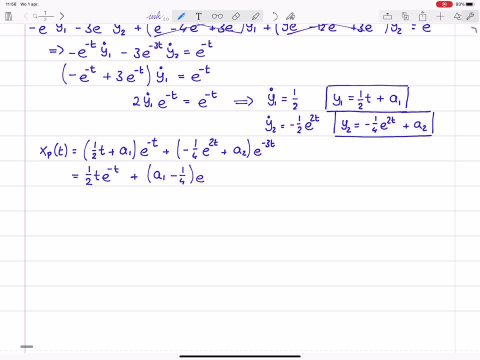 So we have minus 1 over 4, e to the power minus t, and we find just a2, e to the power minus 3t. So we see that the particular solution in this way, using this method of variation of constants, 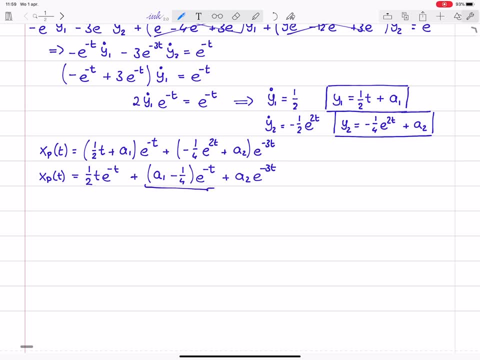 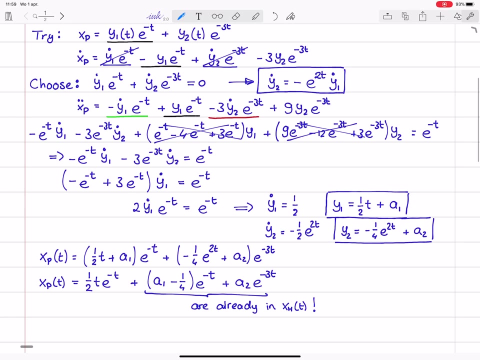 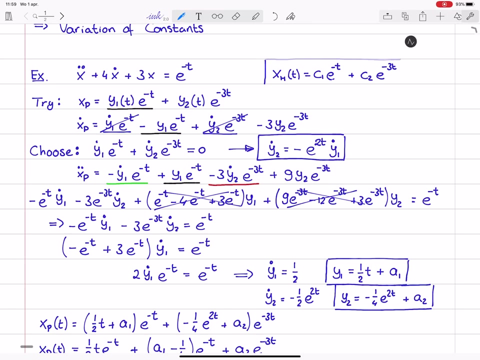 produces two terms, these two terms here that are already in the homogeneous solution. That is important to note. And since the homogeneous solution still contains- let me see where did I write it down? Here it is- It still contains- unknown coefficients: c1 and c2.. 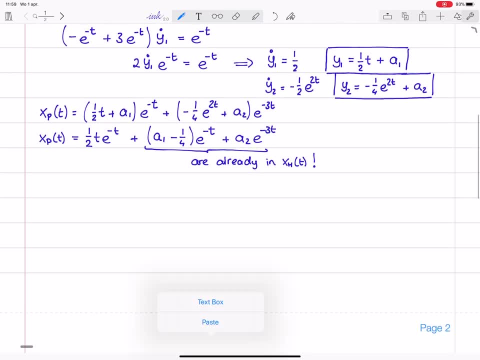 I might as well add these coefficients that I find here to these coefficients. All right, so these- yeah, basically these terms do not produce anything new. This, however, is new. This is really something, a new function, where we see that not only do e to the power. 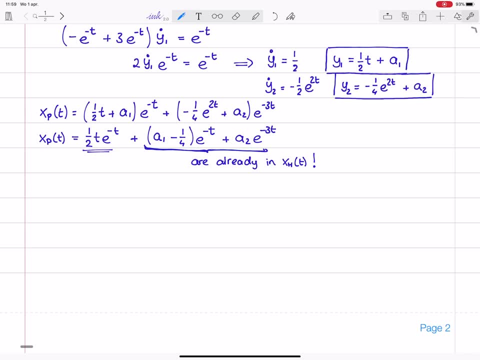 e to the power minus t and e to the power minus 3t satisfy the equation, but also a half times t times e to the power minus t. So that means that the general solution- general solution in this case consists of this homogeneous solution: c1: e to the power minus t.